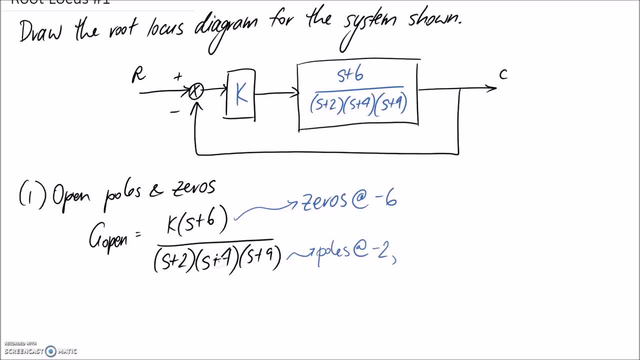 thing: If this here s goes to negative four, then we have the same situation. and here it happens if s goes to negative nine. So we've got one zero and we've got three open loops, So we're going to have two open loop poles. So I'm going to draw our root locus diagram over here, So let's set it up. 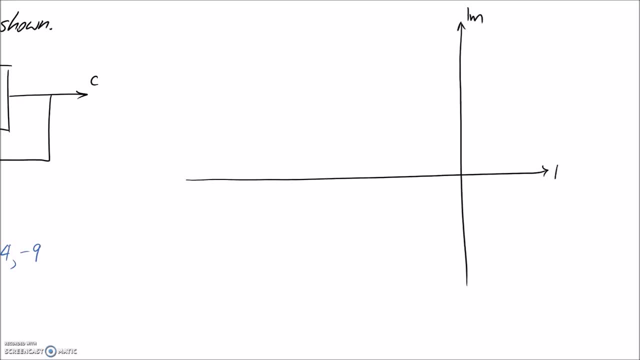 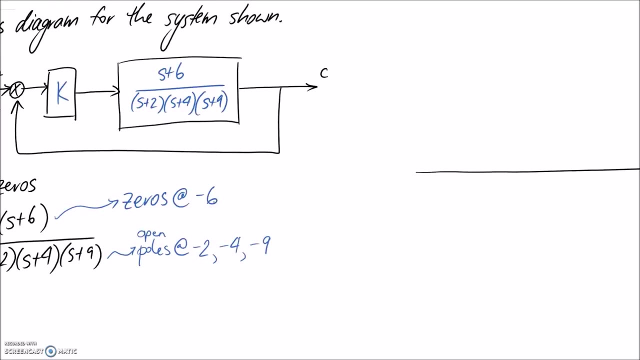 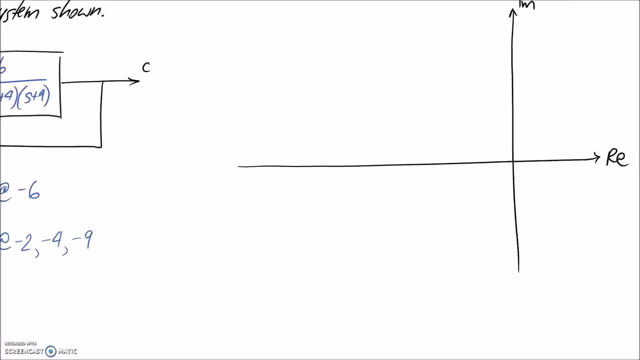 with our imaginary axis and our real axis and we should be able to mark on what we've just identified. So zeros are going to get marked with an o or a circle on the diagram and poles are going to get marked with an x. So we have poles at negative, two, negative four and negative. 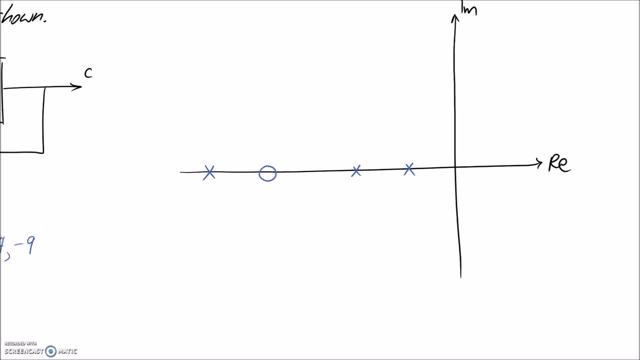 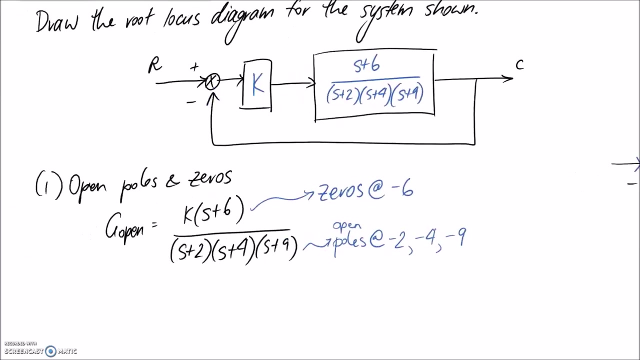 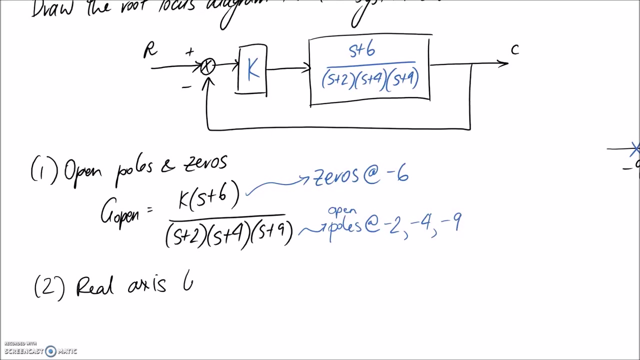 nine something out here, and the zero was at negative six. All right, not super to scale, but anyway we'll do it on MATLAB at the end and you'll see the nice looking version. All right, so that's step one done. So step two is to do the real axis line segments, And for this, what we need to do is: 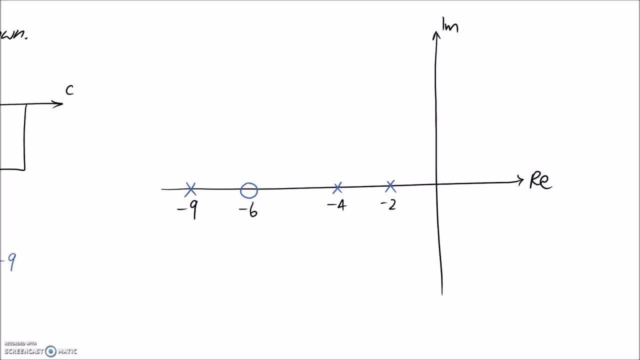 look at our root locus diagram and we're going to have a line segment. So we're going to have a diagram and we're going to join together every second set of poles or zeros, whatever it might be, as we move from right to left. So, starting over here on the right, the first thing that we hit on 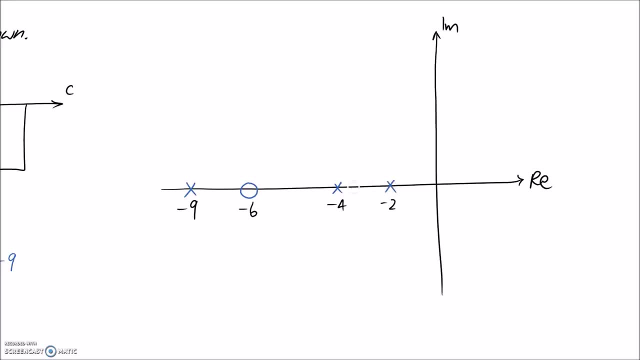 the real axis is this pole at negative two and we need to join it to whatever's next on the real axis. So that's going to mean that these two are joined together and the root locus is between those points. We don't join the next set, so it's blank in here. 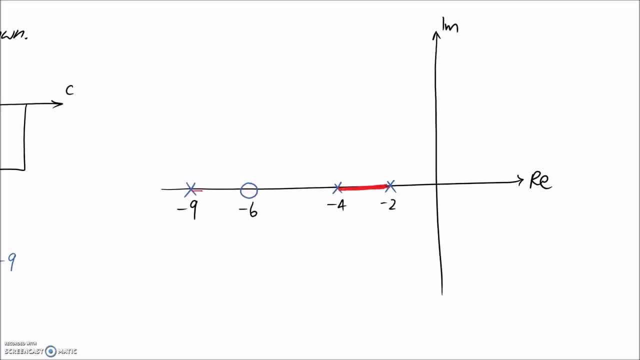 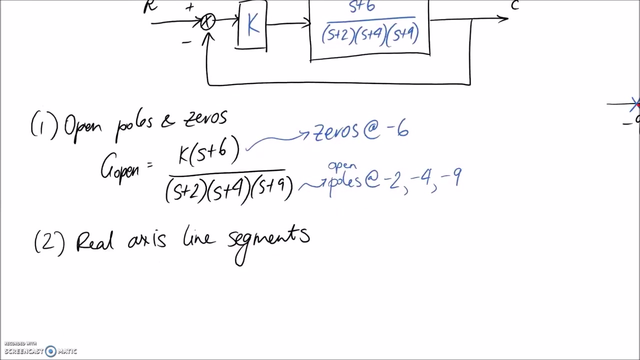 Hit the next one at negative six and we need to join it to the next pairing. Okay, and then there's nothing out here, so that's where it stops. So every second pair gets joined together. All right, so that's been done. So the third thing we need to think about is infinite poles and zeros. 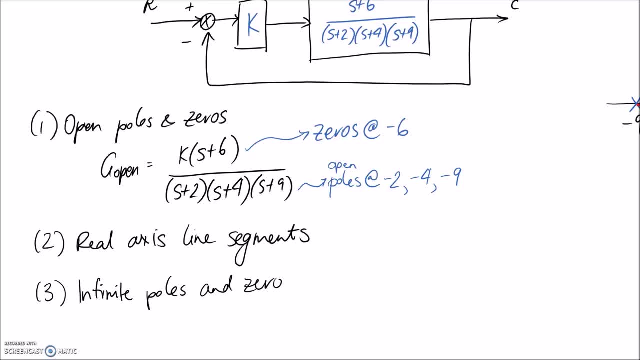 Oops, sorry, and zeros not at zero, So we're going to have a line segment, So we're going to have a. so from before we found that we have one pole, sorry, one zero, okay, at negative six. So the number of finite zeros is equal to one. Here we found that we have three open loop poles, So the number 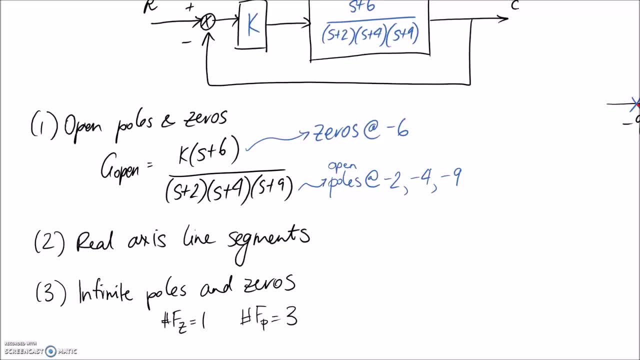 of finite poles is equal to three. So what we know is that the number of poles and zeros need to be balanced within our system, and that's because every pole has to be balanced within our system. Every pole needs to be joined to a zero through the root locus. So in our case, since we have an 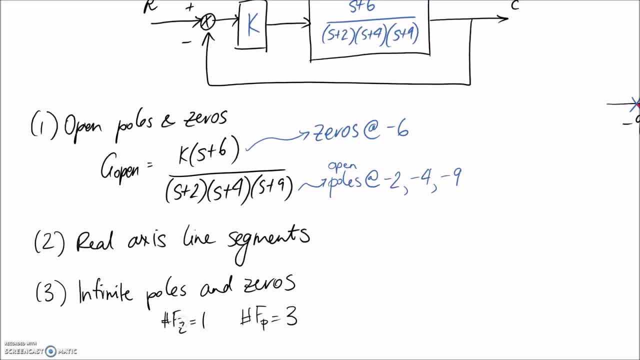 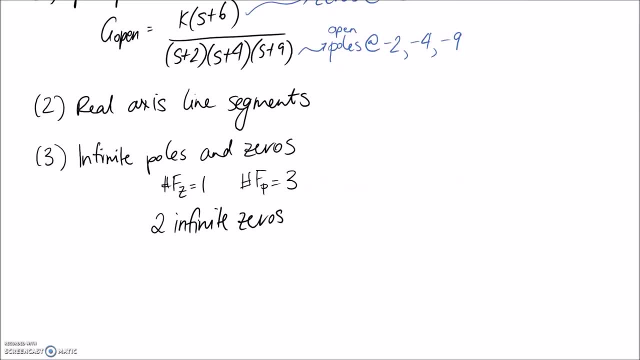 unbalanced number. it means we're going to have to introduce two infinite zeros so that we've got three in total here and three in total here. So I've just noted that in we need two infinite zeros and if we take a look at our root locus diagram we can see where they need to join to. So I said 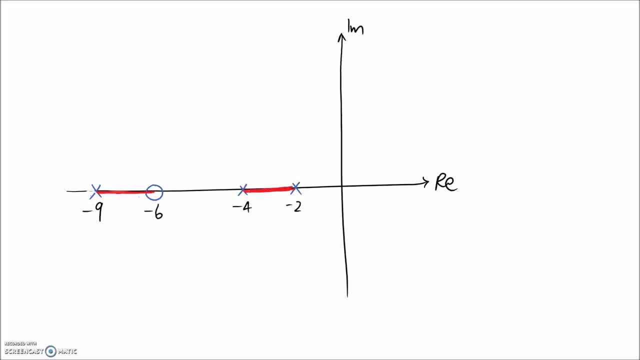 that every pole and zero needed to be connected. So between these two we've already got a connection between a pole and a zero. So we need to have two infinite zeros. So we need to have two infinite zeros and a zero. Here, though, we can see that we've got two poles joined to each other. So what we need to 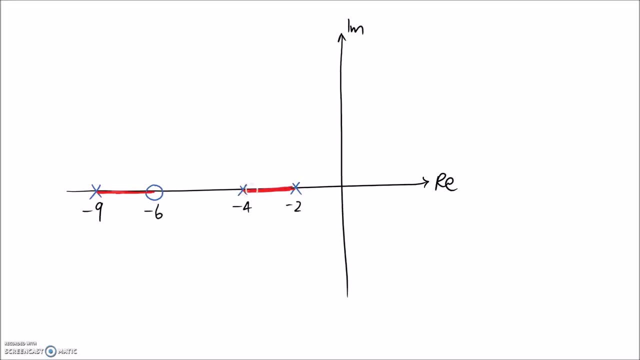 do is introduce these two infinite zeros so that these are then connected, rather than to each other, to these infinite zeros. So when we get a bit further and we look at the breakaway points, we know that we're going to have to have a breakaway, essentially in this area, such that 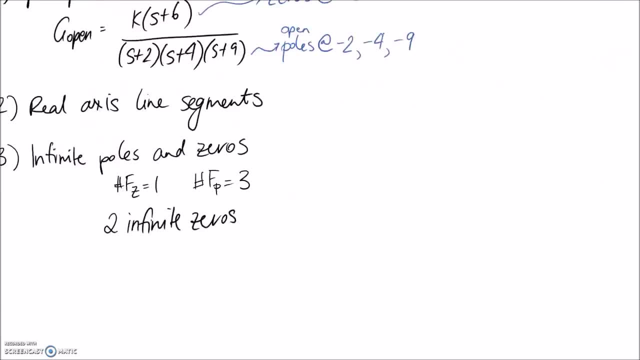 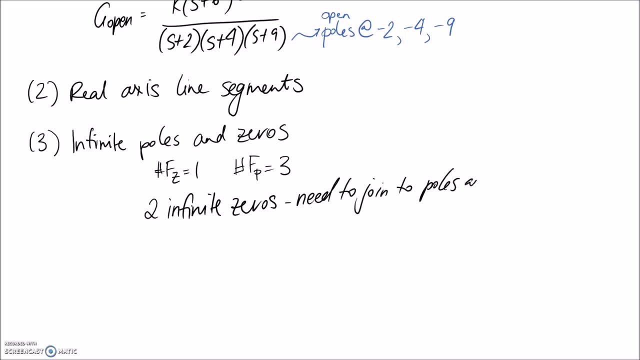 we end up joining the poles to zeros, So let's mark that in. So the next thing that we need to look at now is asymptotes, And we have two equations that we need to apply. The first one is for where it breaks or crosses, I should say, the real axis. 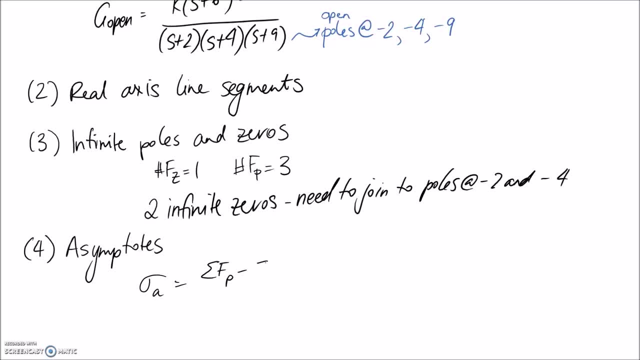 So this is where the crossing happens. So this is where it goes across the real axis. So this is where it goes across the real axis. So this is where the crossing happens. So this is where the crossing happens. this is the equation, All right? so on the top line we have the sum of the finite poles and 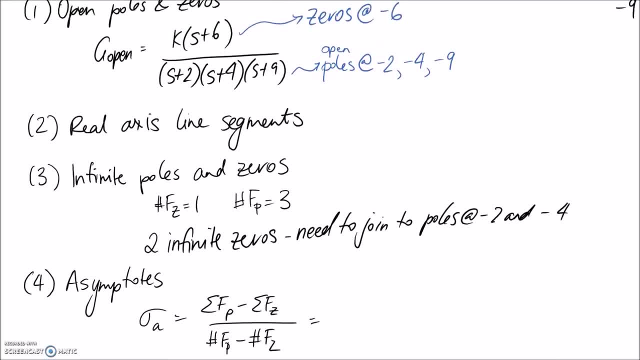 the sum of the finite zeros. So we can sub that in. We have finite poles at these three places, So it's going to be negative 2 plus negative 4 plus negative 9 minus we need the finite zeros, which is negative 6.. So it gets divided by the number of finite poles and zeros. 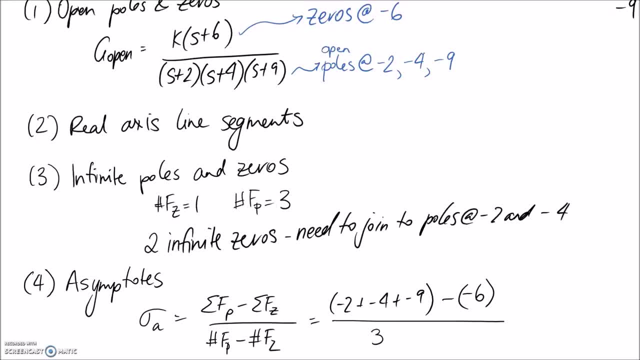 And we work those out as well. We've written them down here. It's going to be 3 minus 1.. So if you put this in a calculator, you find out that your asymptote is going to cross the real axis at negative 4.5.. So the other thing we need to work out for the asymptotes is the angle that. 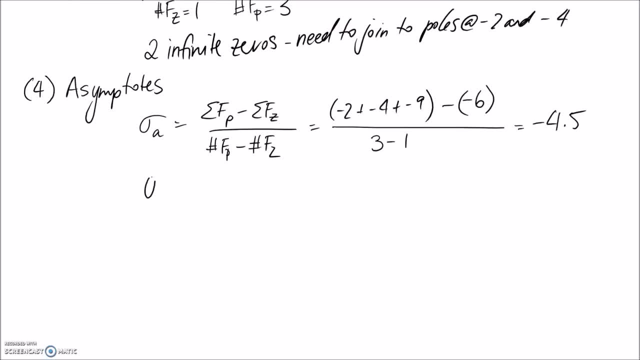 they're going to be at. So we're going to work out the angle that they're going to be at. So, again, we have an equation for that. All right, so what we can do is pick different values of k. k is supposed to be an integer. 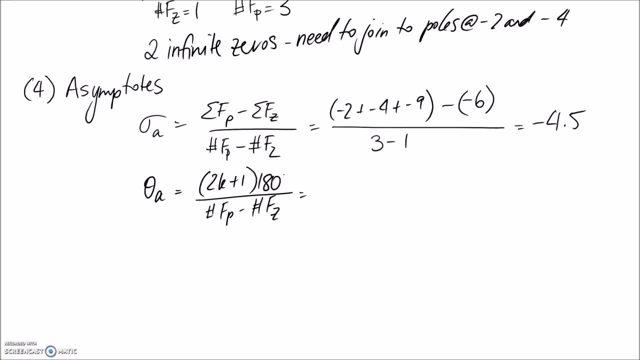 So you can actually pick any integer for it. But I think the easiest thing to do is to start at k is equal to zero and keep increasing it. So we're going to do that. So we're going to do that. So by 1, until you start getting repeating angles. So let's start with k is equal to 1.. Sorry, 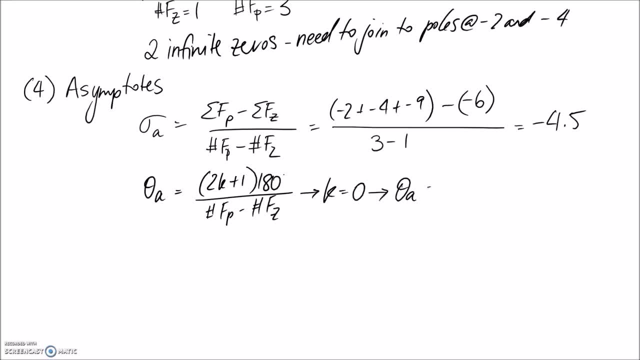 k is equal to zero. That's where I want to start. So if I substitute in: k is zero, that goes away And it's just going to be 1 times 180.. So that's 180 on the top line And the difference between 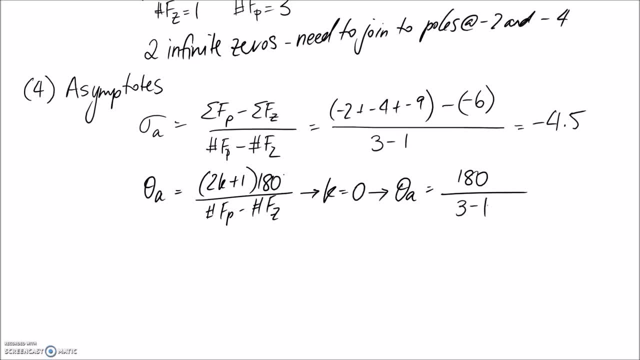 the number of finite poles and zeros is the same as before. We're going to get 3 minus 1.. So this ends up working out to 90 degrees. So let's increase k by 1, and we get k equals 1.. 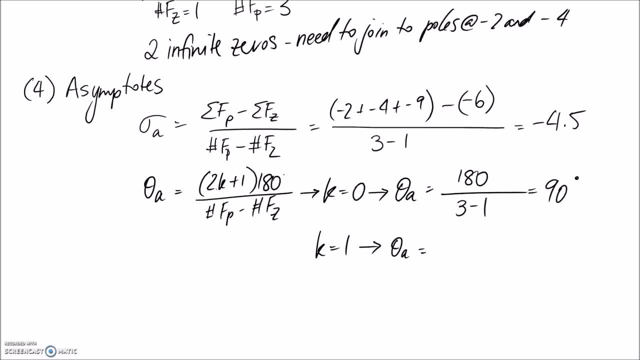 Again if we sum that into this equation. so this time we're going to get 2 by 1 plus 1, and 3. take 1 on the bottom line and this works out to 270 degrees. So if you keep going, say you go, k is equal to 2 now 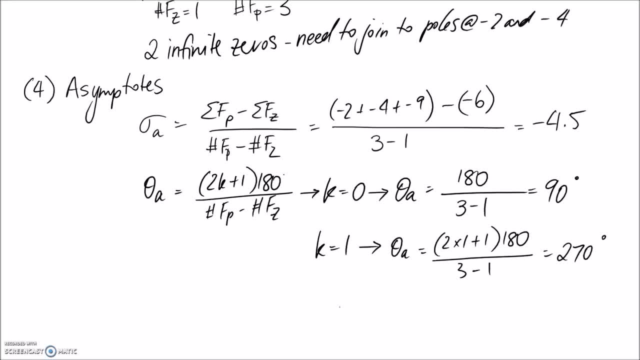 what you're going to find is you end up with a repeating angle, So it's going to be the same as the 90 degree case. So once you start getting repeating angles, you know that you've found all the solutions that you need to for your asymptotes. 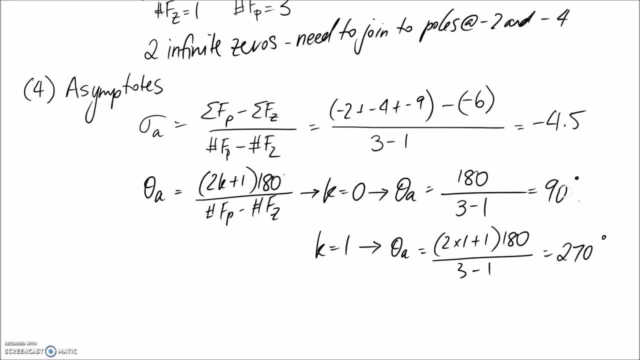 And another way of thinking about it is: the number of solutions that you're going to need is going to be equal to the number of infinite zeros or poles or whatever it is that you need to introduce into your system as well. So, either way, you should end up with the same answers. 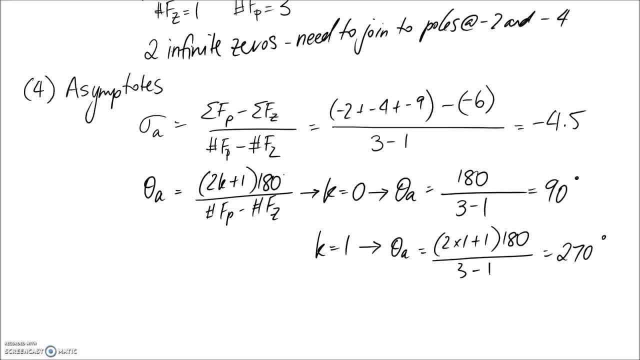 So now we can go ahead and mark these onto our root-locus diagram. So we know that the crossing is at negative 4.5, and they need to be 90 and 270 degree asymptotes. So let's jump over here. 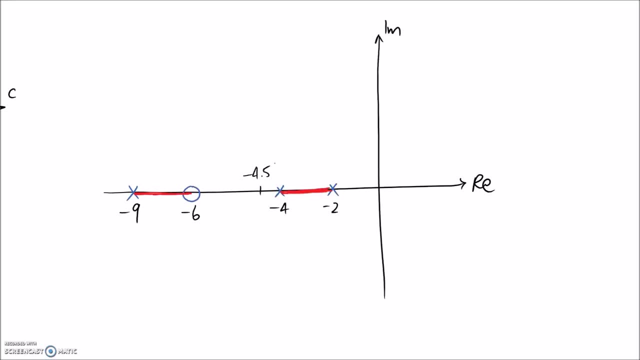 So let's say that negative 4.5 is about here, So we can draw in. we know that it's a straight line asymptote that it wants to approach and it's going to be measuring the angles. So it's 90 degrees as measured from the positive real axis. 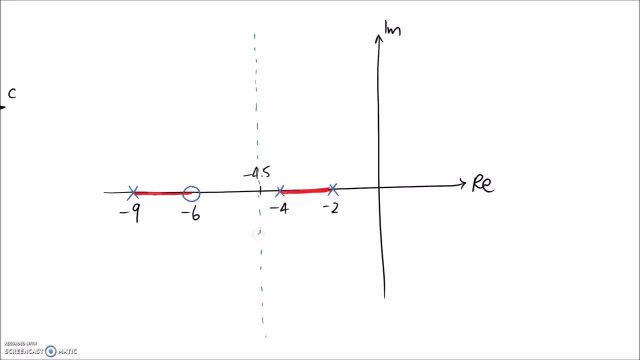 So 90 degrees around to here and then 270 degrees brings us all the way down. So that's why we've ended up with a vertical line that's from the 90 degree asymptote And, you know, going downwards is from the 270 degree asymptote. 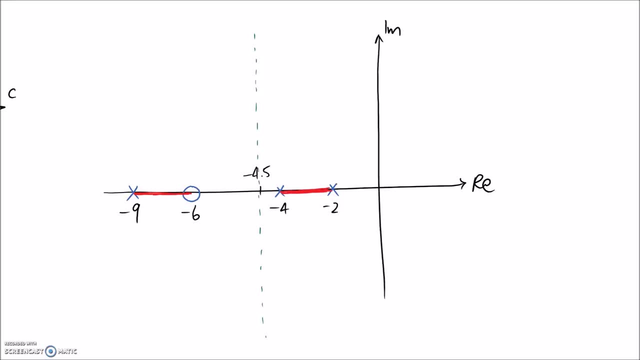 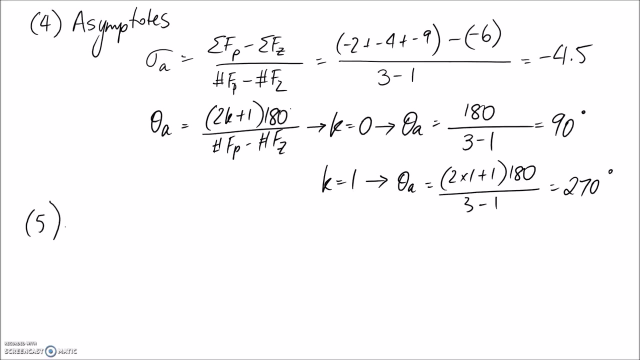 All right. so now what we need to do is work out where our root-locus breaks out of this axis And subsequently then approaches our asymptote line that we've just drawn. So that's step five. So, again, we have an equation for this. 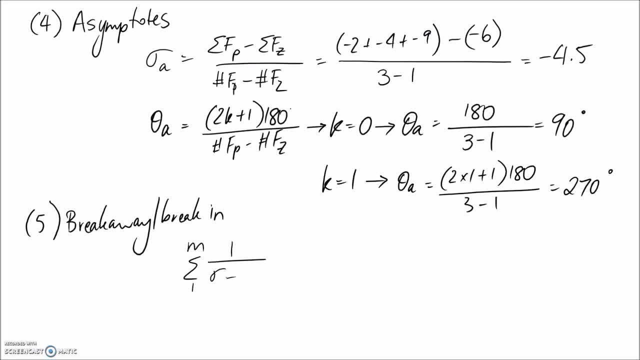 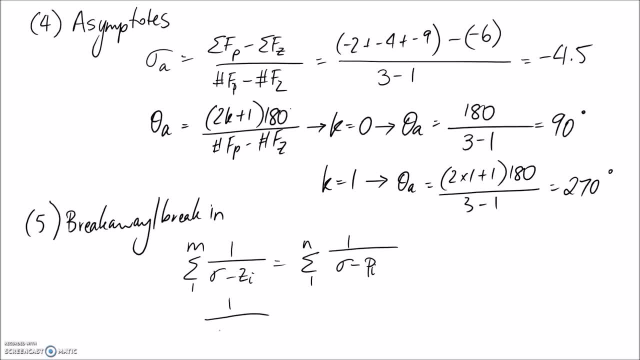 So, putting this in, we had a zero at negative six. So this is going to end up being a double negative, so it becomes positive six, And then we have three poles that we need to put in here, So we had one at two. 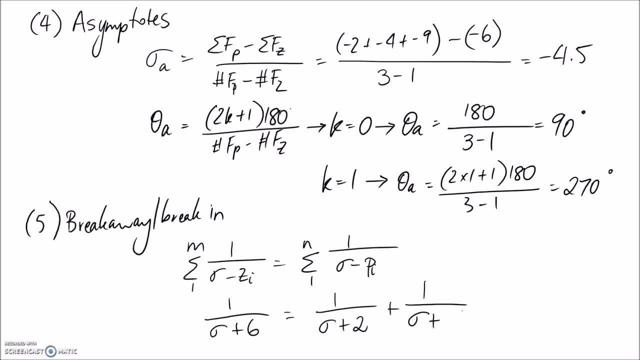 It's a sum of so we add on. We then had a pole at four, another pole at 9.. So this equation here is really ugly to try and solve by hand, because it ends up being a polynomial and it's going to be a third-order. 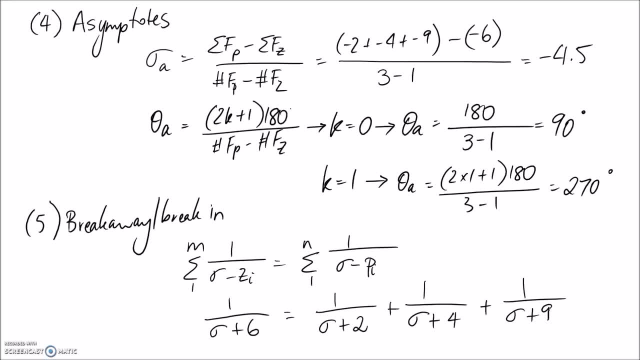 polynomial, so it's a bit messy. So what I'd recommend is, in this situation, go ahead and put it in MATLAB or Warframe Alpha or your calculator to be able to solve it. So I've put it in Warframe Alpha. This is it, and it's given me three. 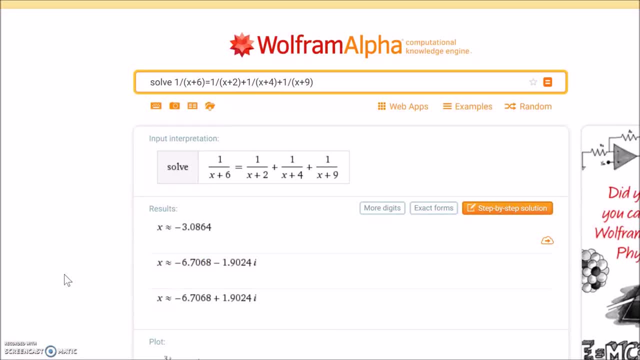 different solutions to my problem, so I'm going to need to go ahead and figure out which one is the one that makes the most sense. So let me just put these down on our paper, our three solutions. Okay, so, looking at these, only one of them is: 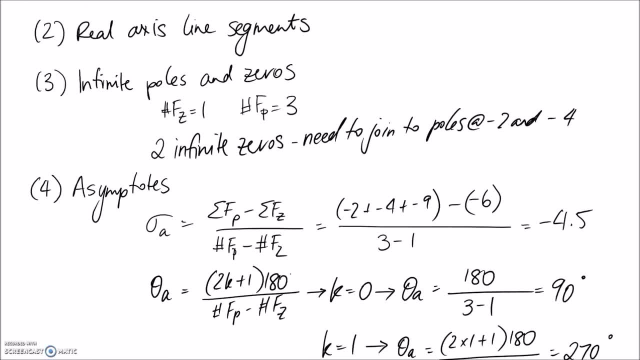 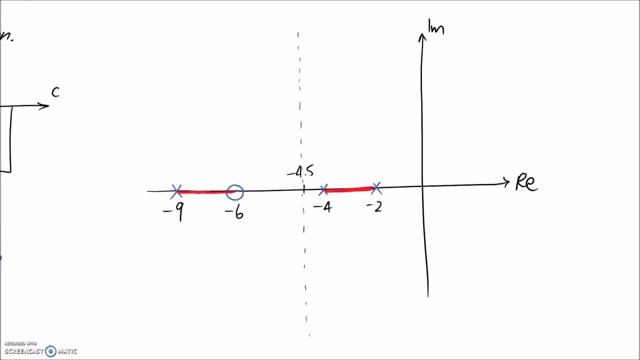 actually going to make sense. So before up here at step 3, we concluded that we need two infinite zeros and they need to join to our poles at negative 2 and negative 4.. So we can see that these are joined along the real axis. so it only 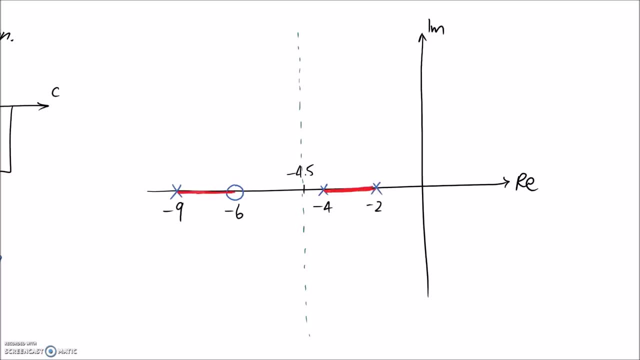 makes sense that our breakaway point can sit on that axis. So two of the solutions that we just solved for actually had imaginary components, so they'd be sitting up somewhere off the axis and doesn't make sense. So we need to pick the real number. that's between 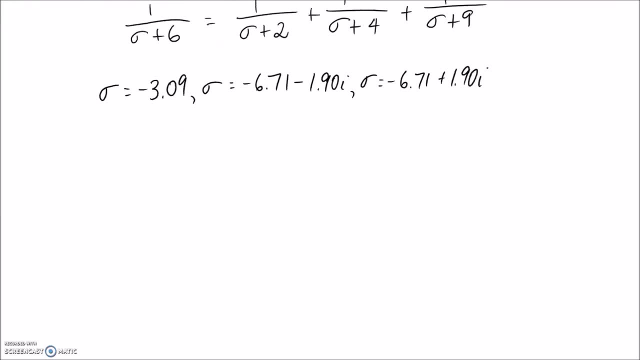 negative 2 and negative 4.. So if we pop that back down, this is the one that's going to make sense. It's between negative 2 and negative 4 on the real axis. These ones don't make sense, so we can discard them. So let's go back up. 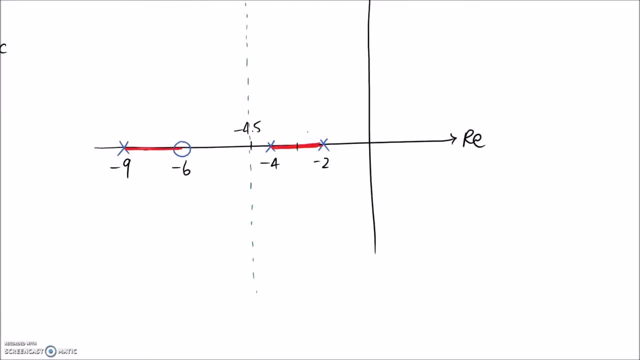 here and mark in. So we'll say about: here is our negative 3.09.. So that's where it's going to break out of our axis. So we should be able to complete the root locus now. So when it breaks out of this axis it needs to break out at 90 degrees up and down. 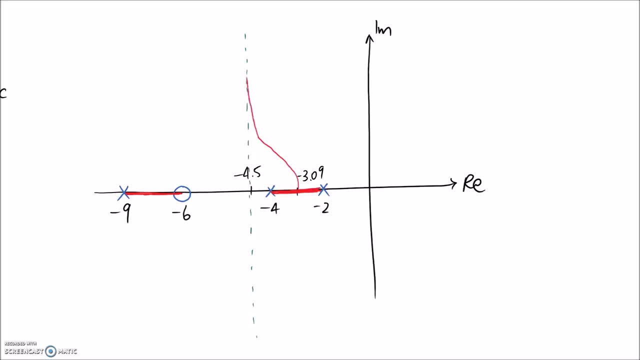 It's then going to try and approach this straight line asymptote and it gets closer and closer to it until it actually touches it At when it reaches infinity, positive infinity and negative infinity. So that's my best job of drawing it manually. If you want to, you can try and compare. 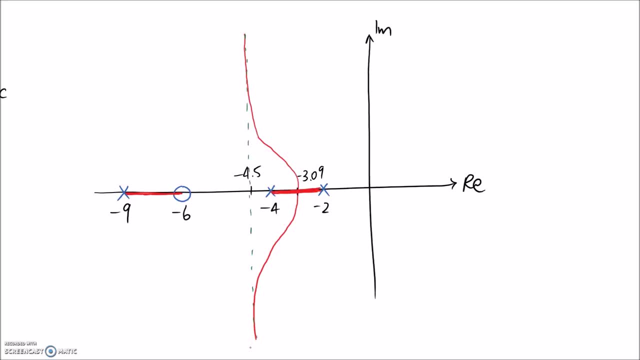 against the MATLAB one, which we'll do in a second. So there was one last step to our process for drawing these root locus diagrams, and that was to find the imaginary axis crossing. Now we can actually look at this root locus diagram and see that at no point is any of the root locus coming. 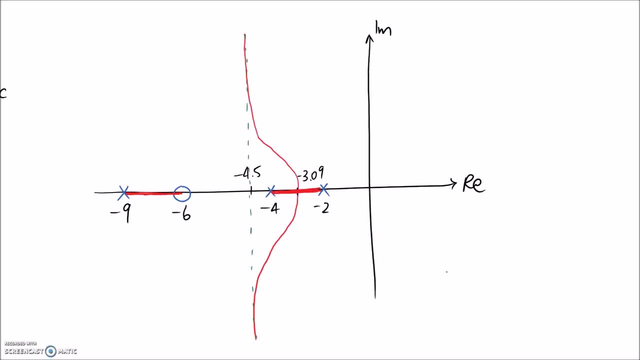 across this imaginary axis. So therefore, there's no point trying to compute where that happens, because you're not going to get an answer that makes any sense. So this is our complete thing, and let me just mark down the bottom here, Step 6.. 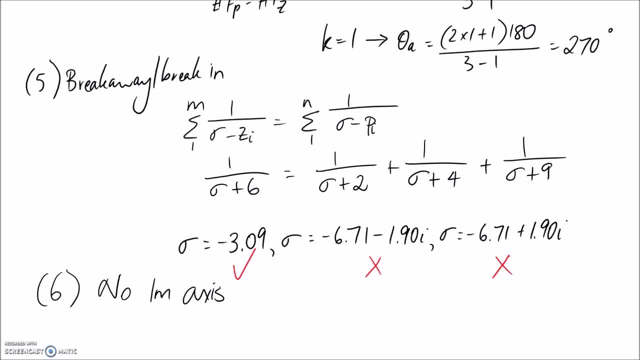 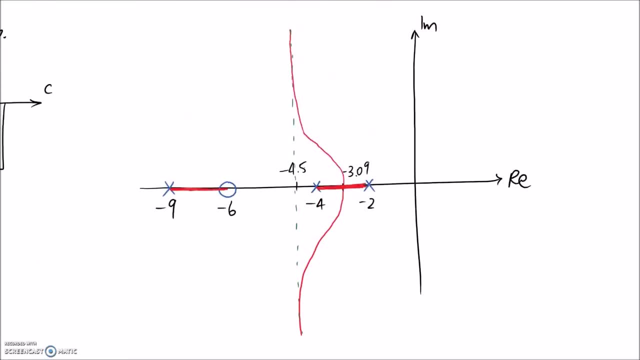 We've got no imaginary axis crossing, Alright, so let's compare my solution with the MATLAB one, because MATLAB is obviously going to be able to draw much neater than me. So that's ours. If we have a look at MATLAB, this is the code that I wrote to: 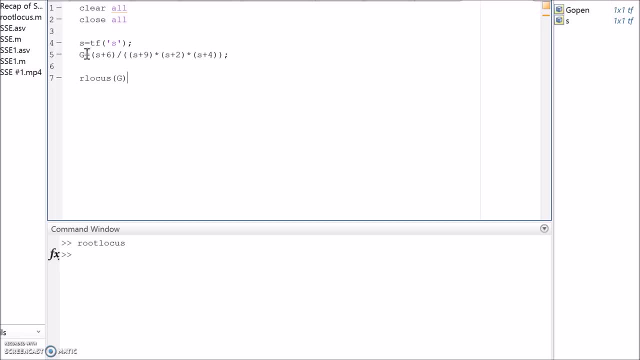 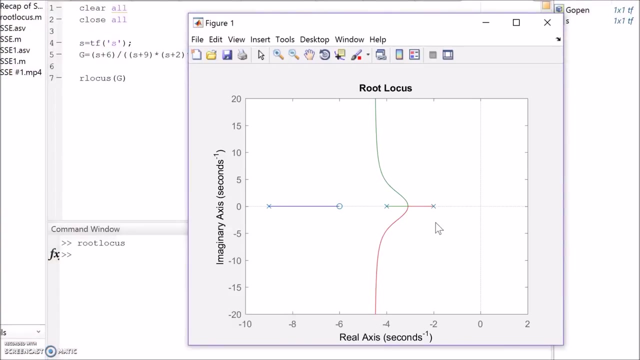 be able to look at it. Just remember that you're looking for the open transfer function in here and you don't put the K inside your transfer function for MATLAB, because when you plot the root locus, MATLAB is going to do that for you. So this is what it plots and where these lines move. that's telling you where the 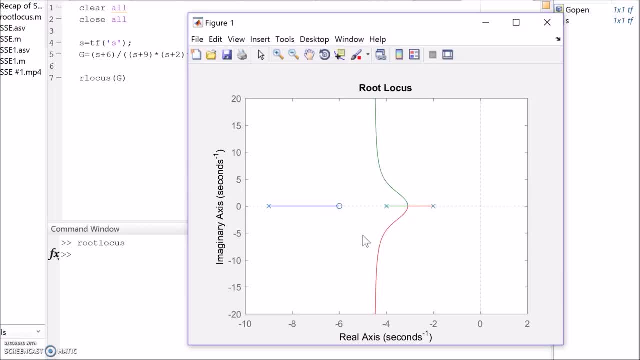 poles and the zeros are going to go as you change your K value, So we can double check our values that we got. So one of the critical points that we saw was the breakout point for our root locus. So if you drag your point down here, you can. 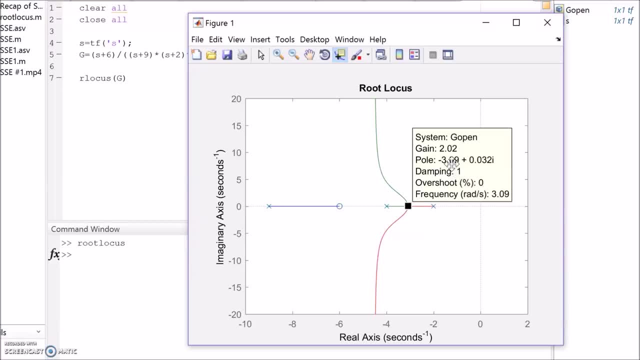 see, this is as close as I can kind of get to where the breakout occurs and we can see it to negative 0.39.. sorry, negative 3.09.. For the real component, this is almost zero, so it's pretty much on. 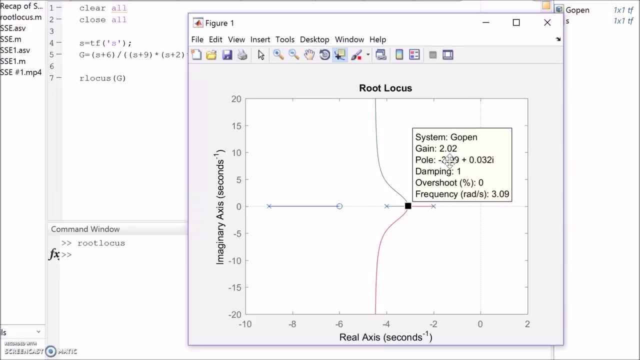 the spot And that agrees with what we calculated for the breakout point. So the other thing that we can look at is what value our two branches here approach, because that's going to be the asymptote line. So if we go as far as we can on this diagram,